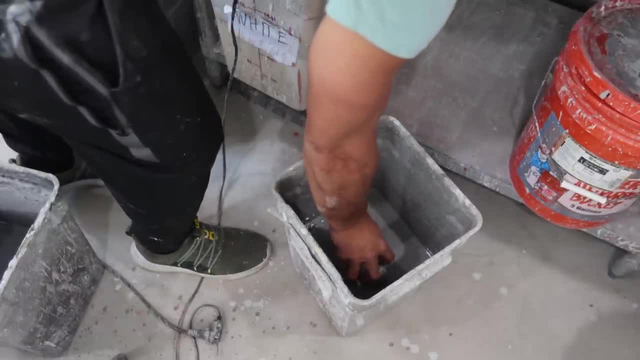 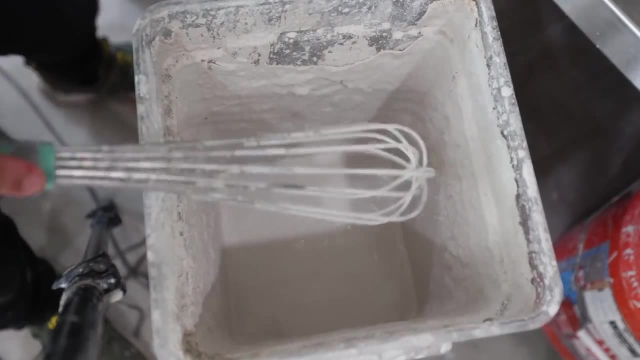 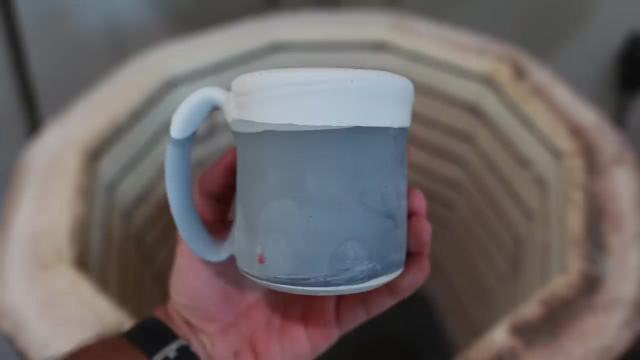 I haven't been glazing this one in a while, so that's really unfortunate. I knew that was going to happen too when I was glazing it. it just seemed so bad. I haven't been glazing this one in a while, so that's really unfortunate. I knew that was going to happen too when I was glazing it. it just seemed so bad. I haven't been glazing this one in a while, so that's really unfortunate. I knew that was going to happen too when I was glazing it. it just seemed so bad. I haven't been glazing this one in a while, so that's really unfortunate. I knew that was going to happen too when I was glazing it. it just seemed so bad. 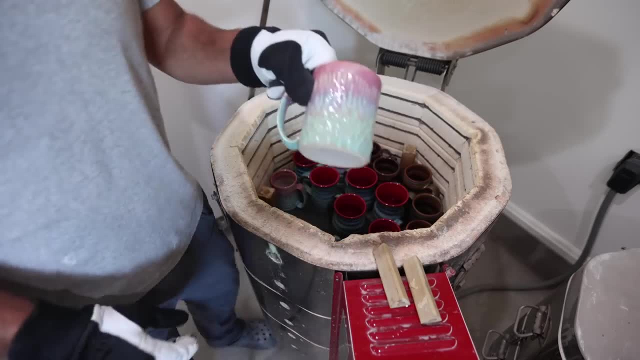 I haven't been glazing this one in a while, so that's really unfortunate. I knew that was going to happen too when I was glazing it. it just seemed so bad, super thick. We got that one That looks really nice. Raspberry Mist, Alabaster and Norse Blue. 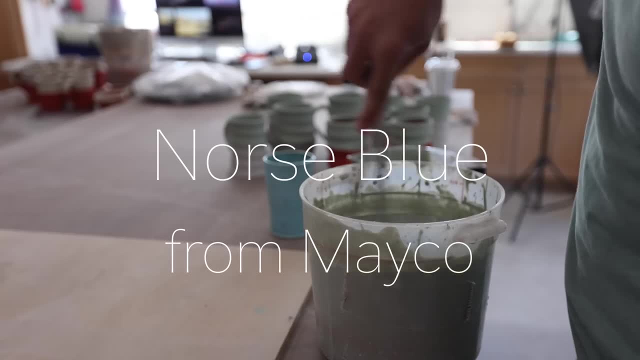 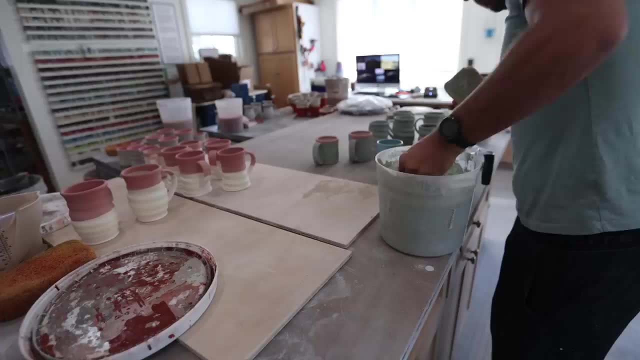 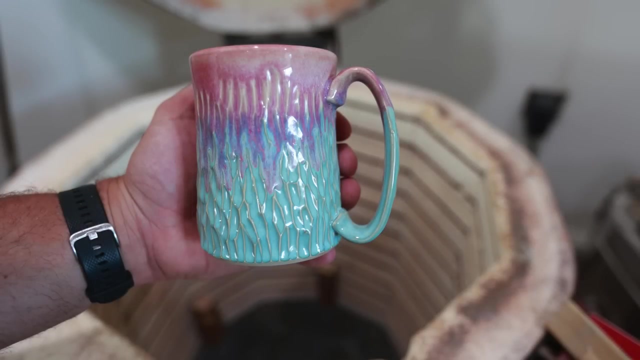 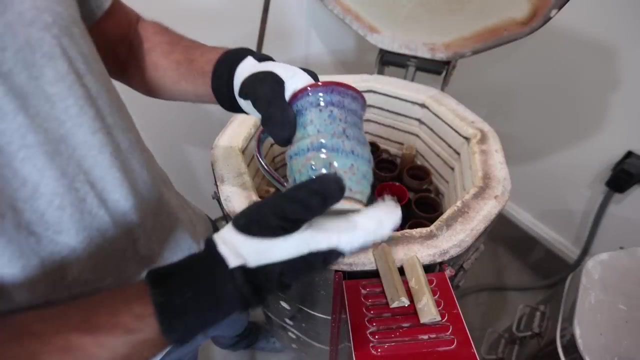 That's the same combo right there, just not on a carved mug, All right. and then the next combo that I show you: Aurora Green over Bright Red, So basically Bright Red on the whole thing. and then Aurora Green over Light Red. So that's the same combo right there, just not on a carved mug. 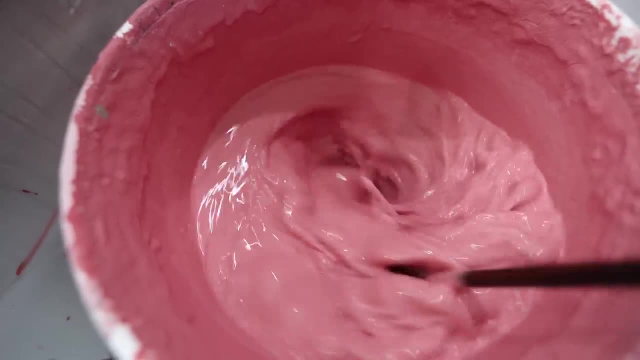 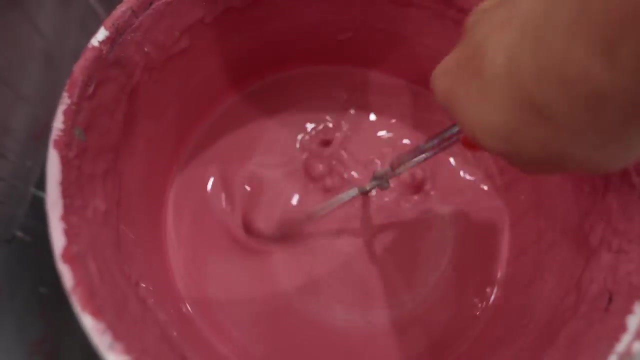 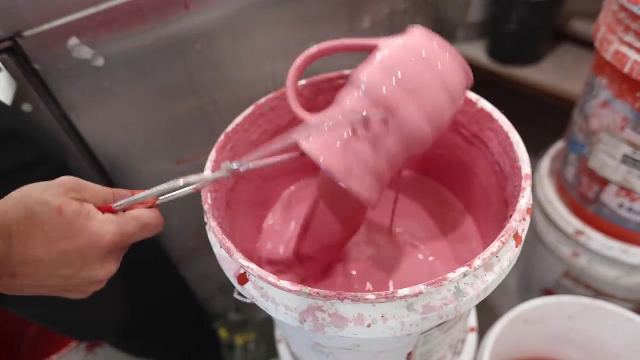 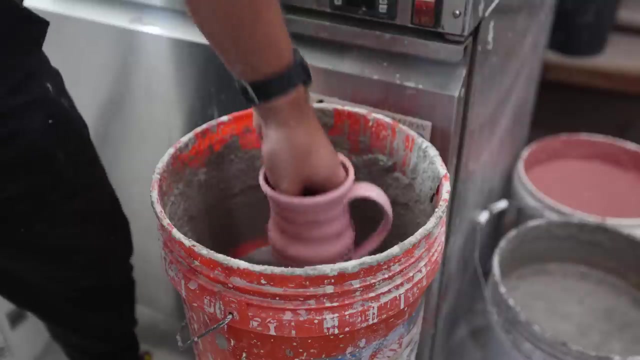 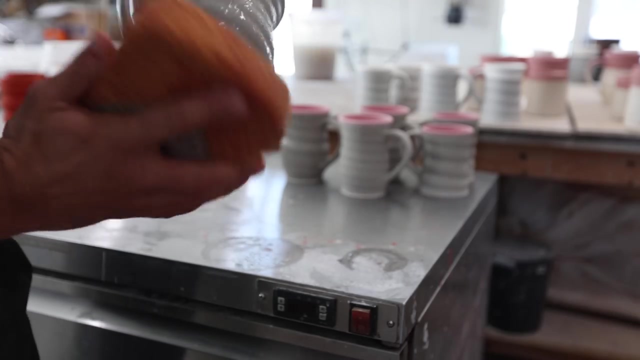 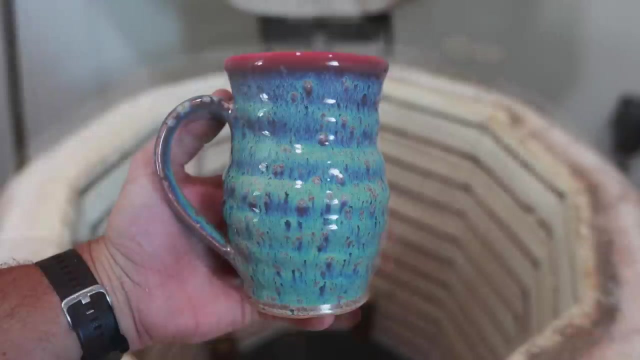 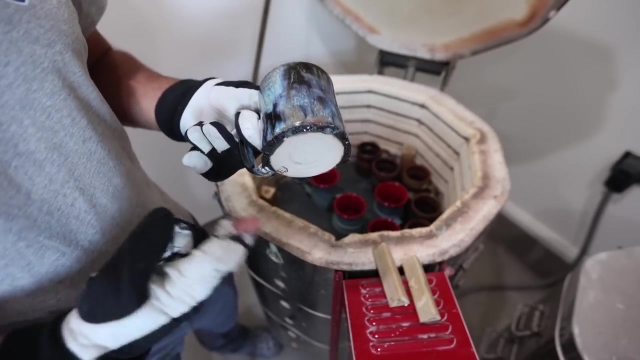 Left on the outside. That has become one of my favorite combos- Has sold well, Wow, that is like I haven't had a drip that bad in a while. I think the black is too thick. I think the metallic green is too thick. 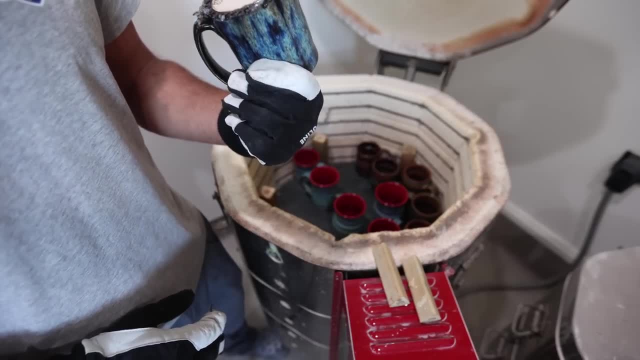 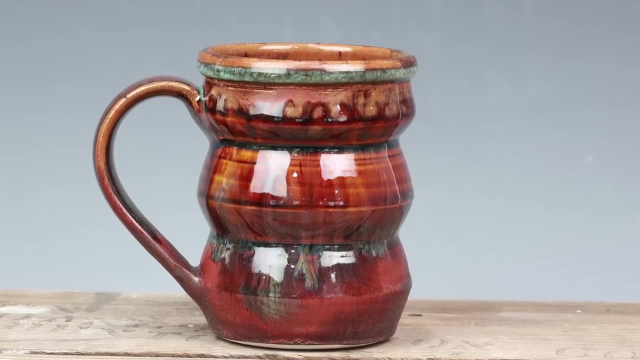 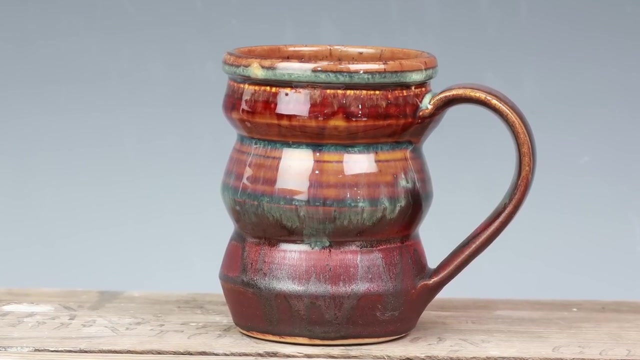 Look at that. That is like real bad. Okay here, No, that's really nice, Dripped a little bit, but salvageable. Norse Blue, Norse Blue over Copper Ore. Also Norse Blue over Copper Ore, That's really love it. And then the. 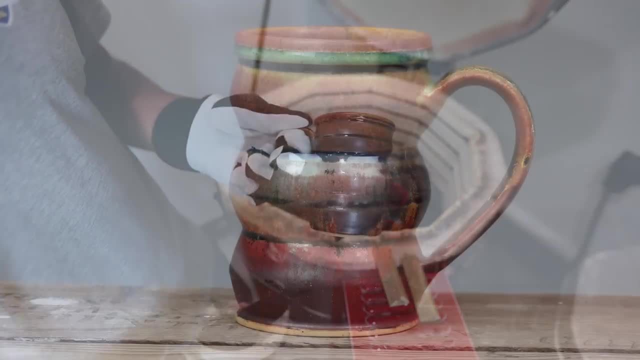 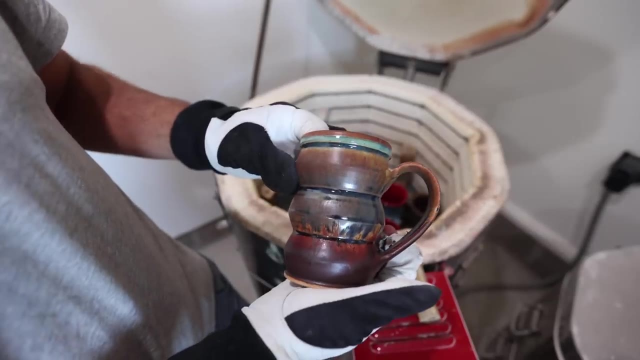 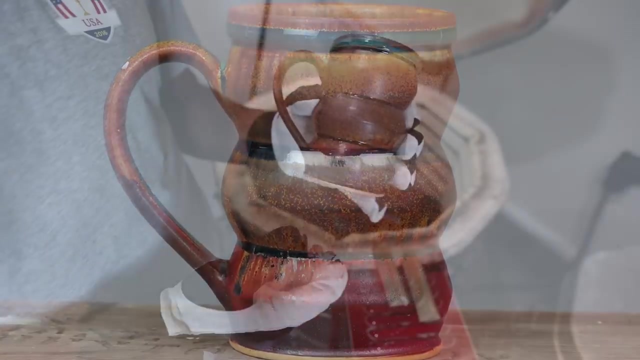 best new combo: Desert Sunset- Whew, sweet, It's pretty epic, Pretty epic. looking right there, Boom, love it. Look at that How it's like kind of green up here with the orange and the copper. Wow, beauty. And it's just super consistent Like it always is coming out really nice. 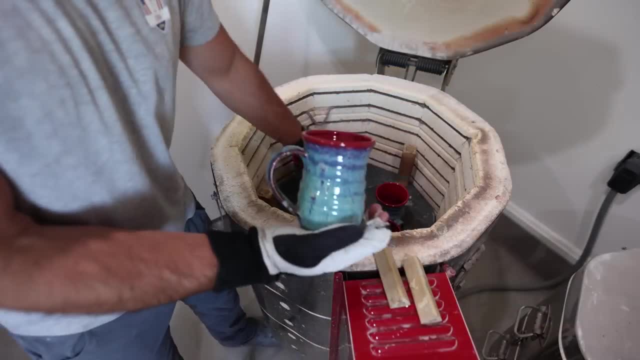 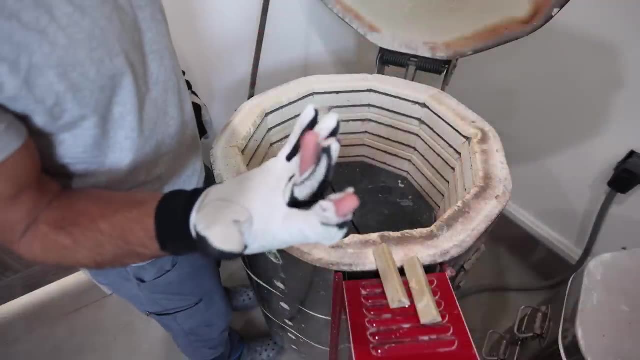 Cool, cool, cool cool. All right, then I've got a bunch more Roar Green over Red. Wow, that's really nice, Really nice. Like my gloves they don't work too well. Noice, Not quite as bad of a drip as was in the earlier. 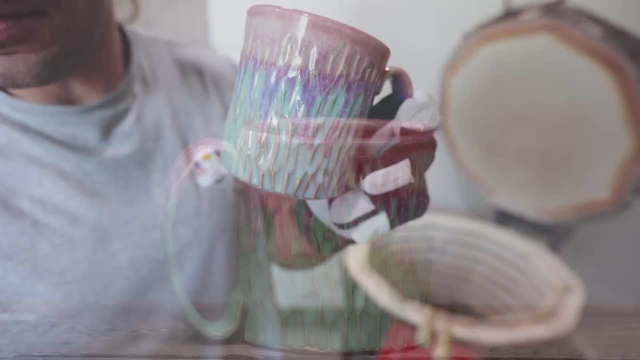 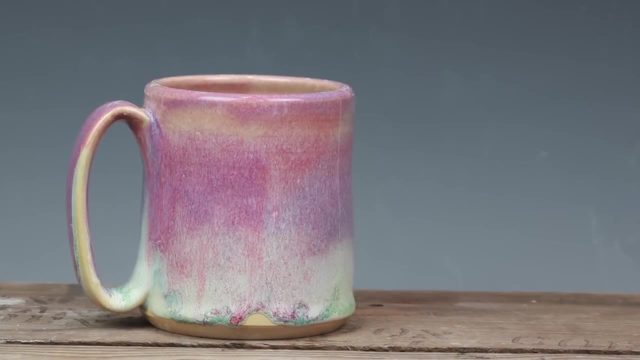 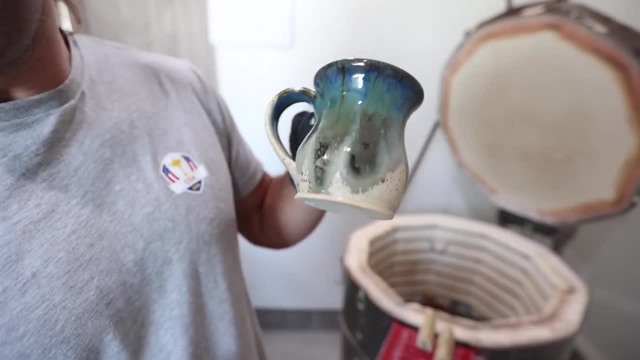 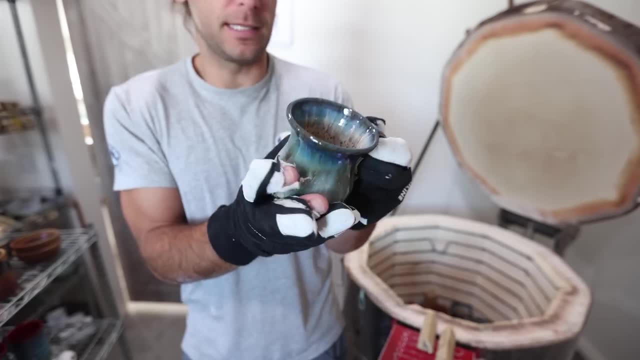 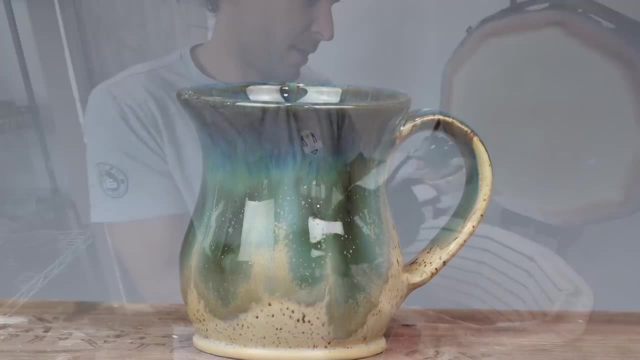 and so then I'll glaze it again and then flip it over and glaze it upside down, and that's what the Insanity is. but sometimes these ones just turn out really good by themselves, In which case I don't. but if I see any pin holes or imperfections, then I'll reglaze it. 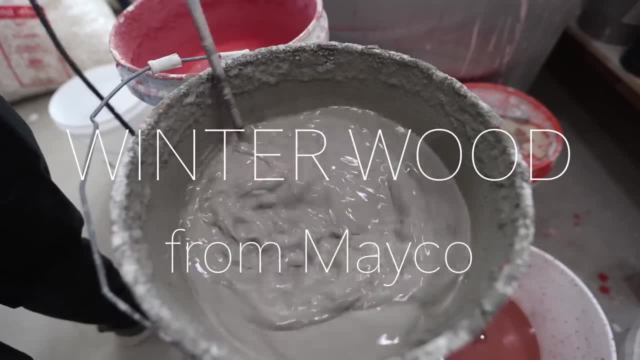 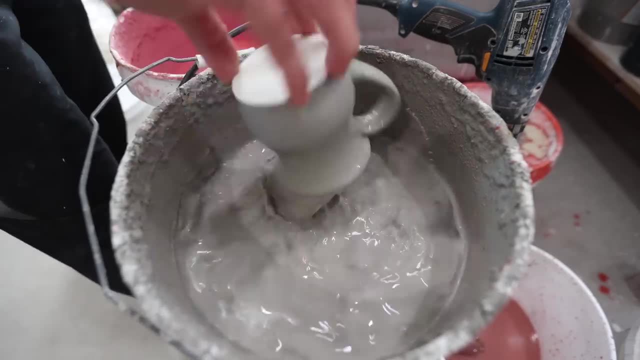 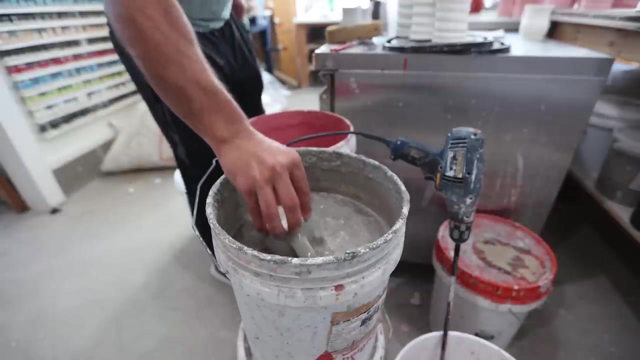 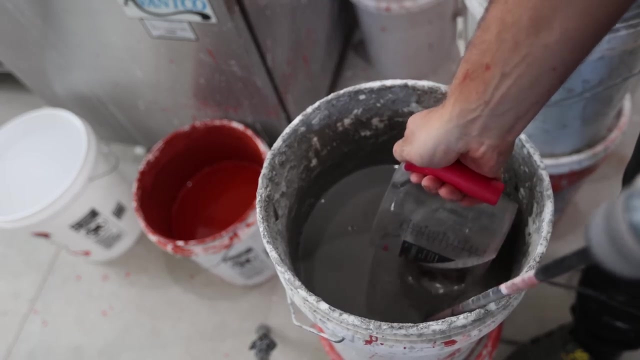 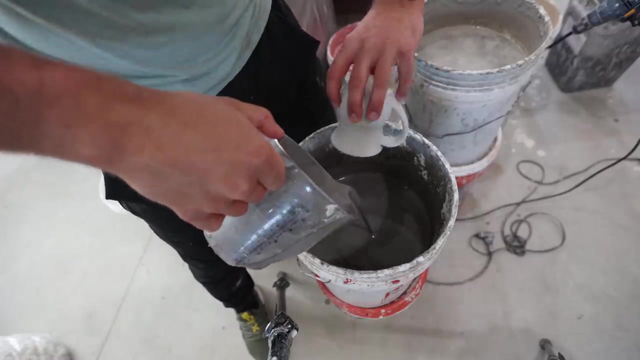 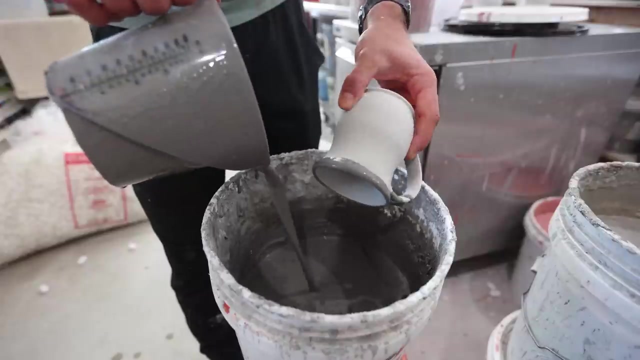 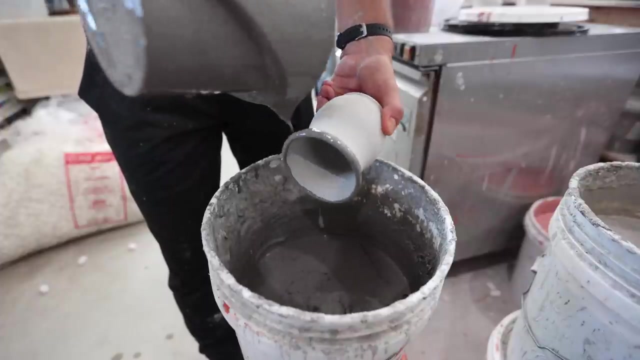 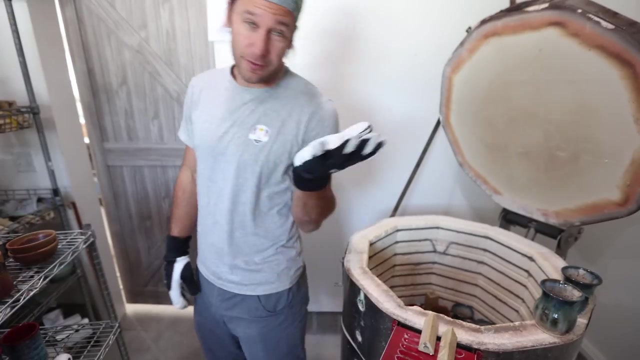 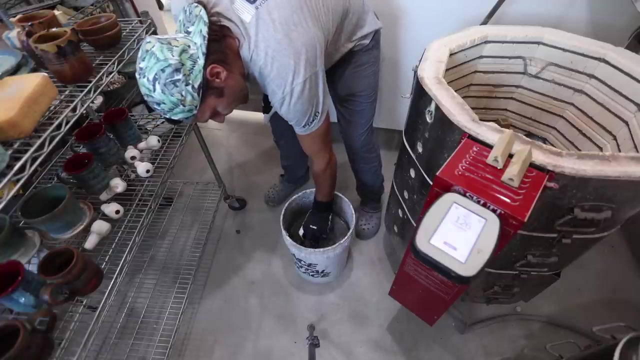 Put it back in the kiln. Okay, so I'll get the Midnight Rain and I'll do it right now, because if I glaze it right now, then while they're still pretty warm, then the glaze will dry quickly, Half in to overlap, like that. 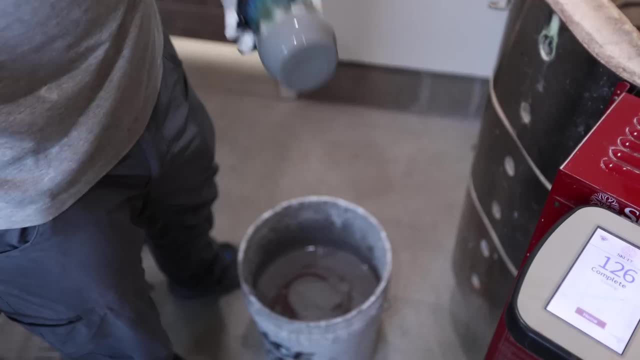 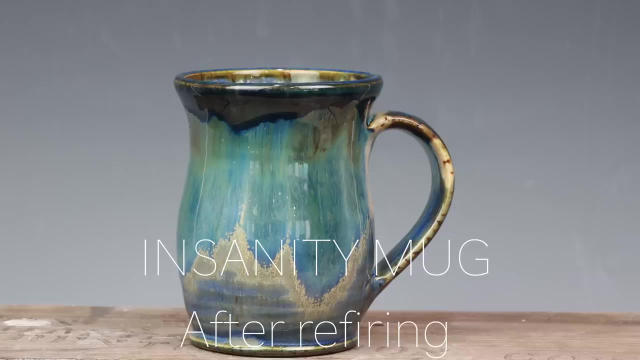 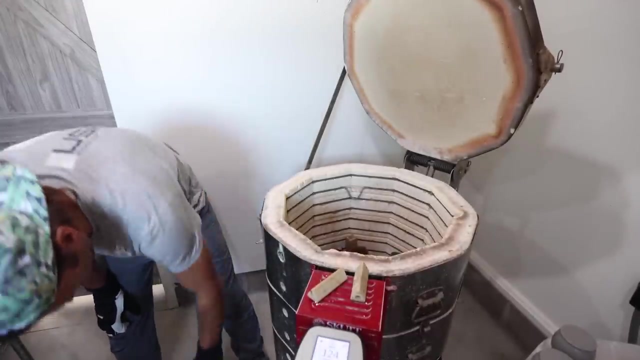 So now the bottom is glazed like that and then it's warm, so it should dry pretty quickly, And then I'll refire it upside down with a little stilt. All right, okay, then I'll pull out these next two Pinhole so that becomes an Insanity and it's just like one little tiny pinhole. 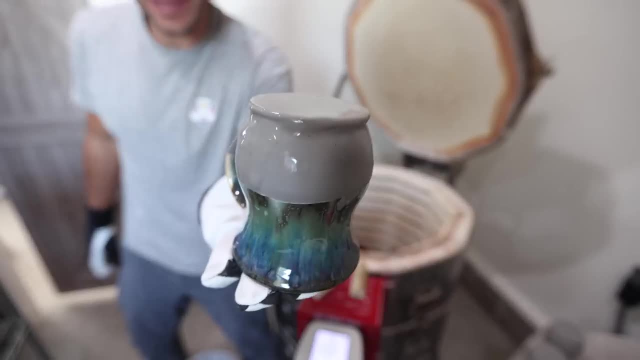 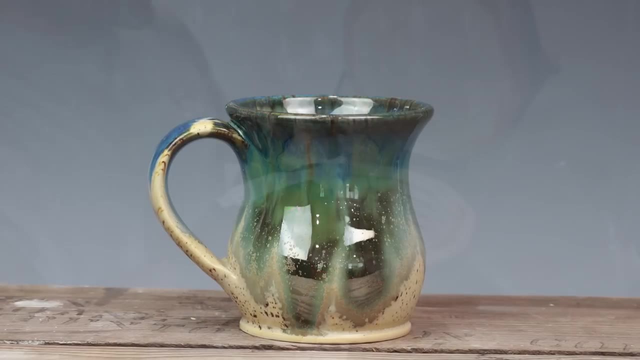 I just like those Insanity mugs too. So then they'll get fired again, just like that. So there's three that'll become Insanity mugs, Two that are not, And then this one. it's really good. I don't see any any issues at all with that one. 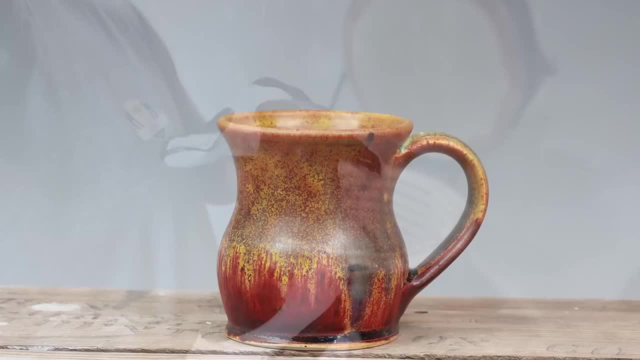 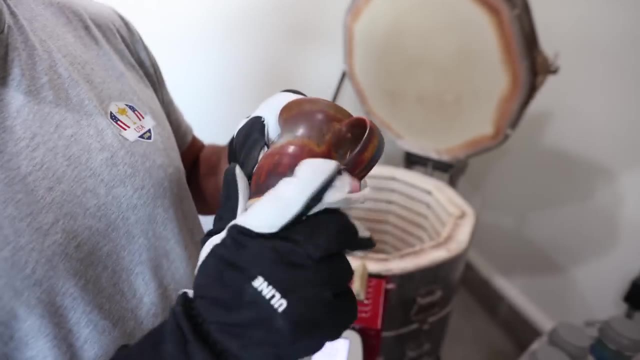 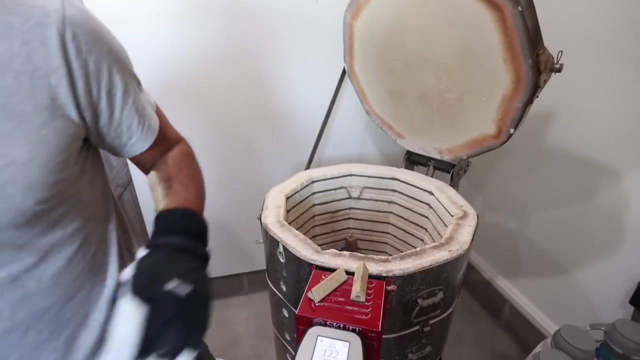 All right, yes, look at that, Holy cow, that's so good. So, oh, just so good, Love it, love it. Boom, coming out hot, No pun intended, the best I probably have, 12. The 15 of this glazed combo for sale in this restock. 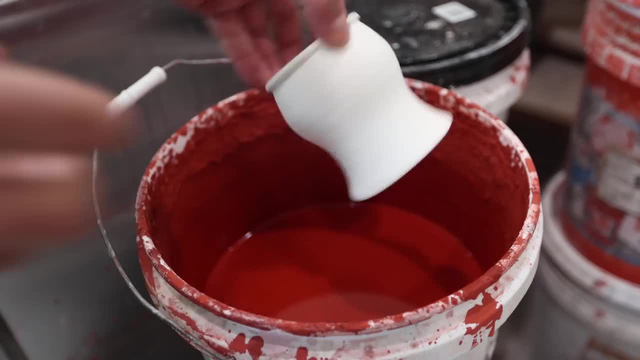 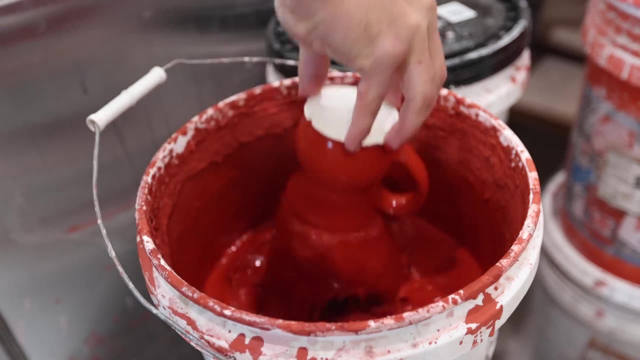 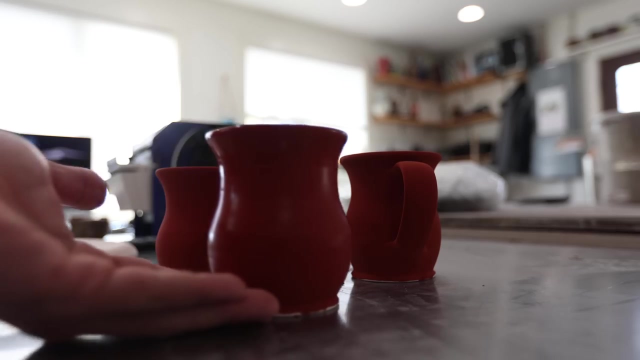 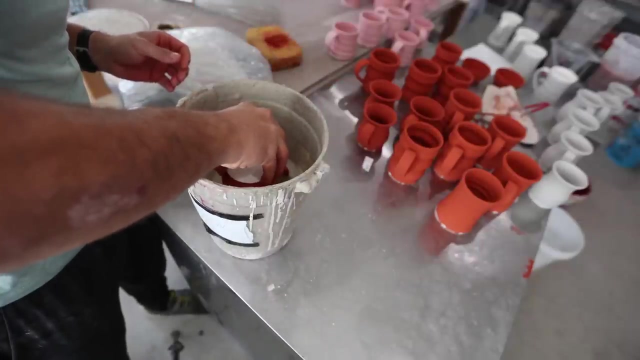 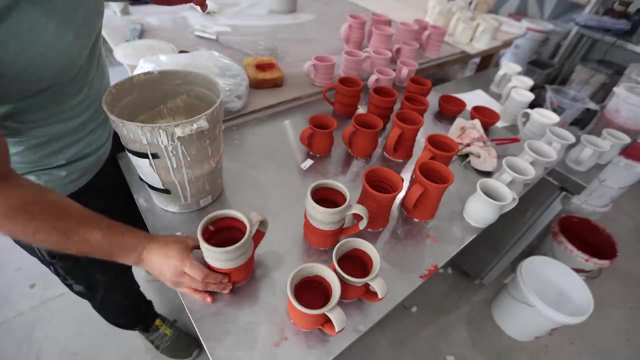 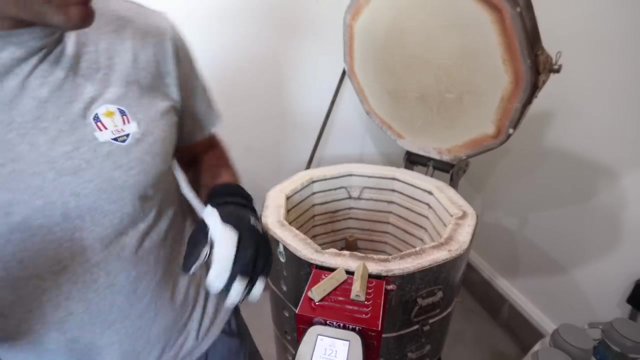 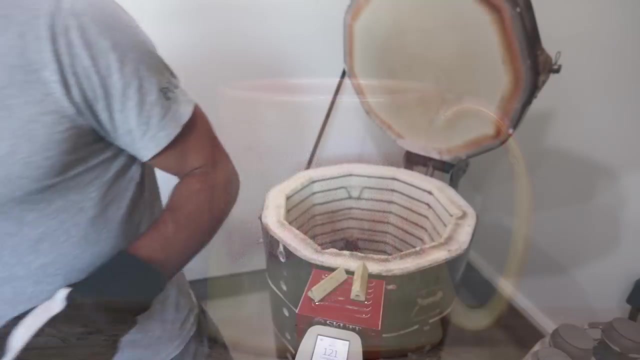 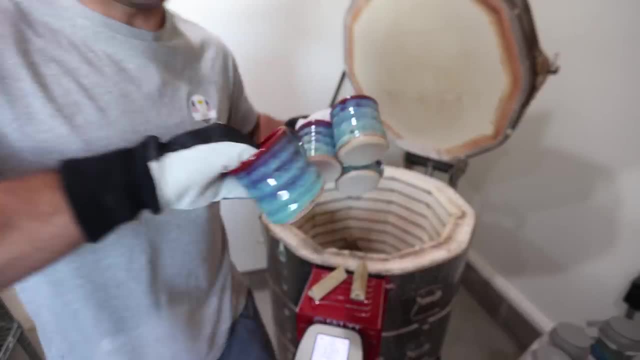 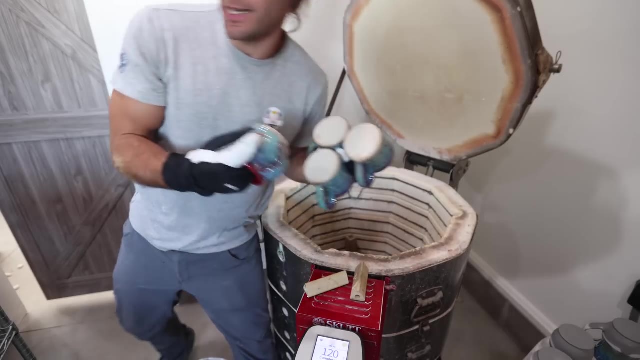 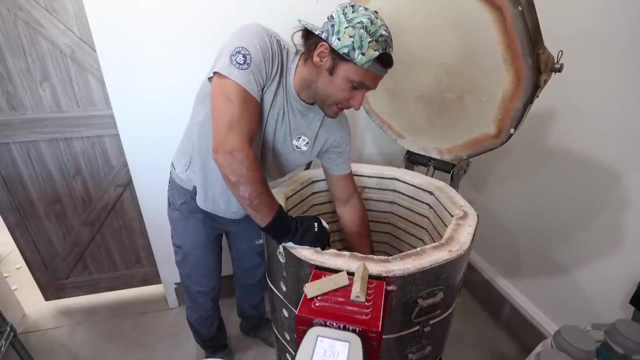 Got a bunch of those, Not a really popular combination. Funny part about this combination: I can't put it at the bottom of my kiln, the bottom shelf. It turns out different but So whenever I fire that glazed kiln or that combination I always make sure that it's on the next shelf up. 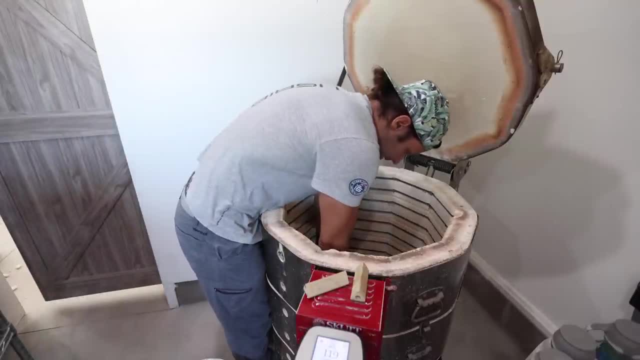 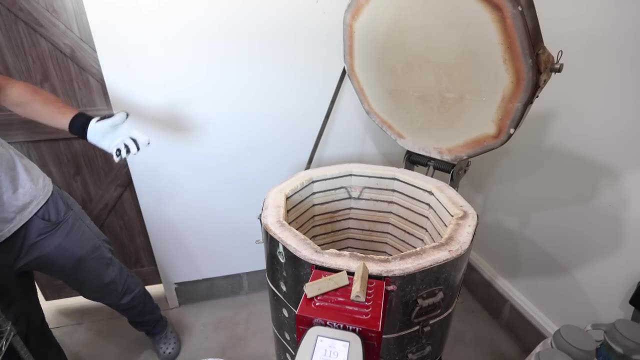 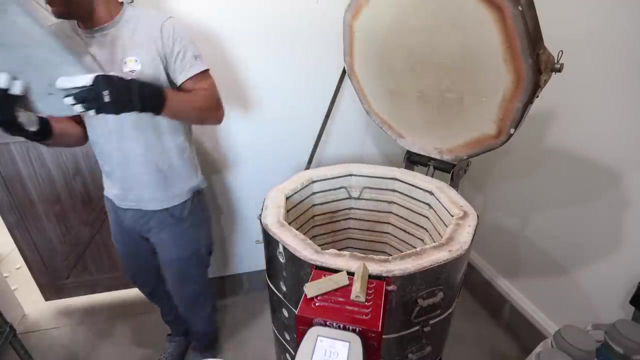 It's funny how certain combinations work differently at different parts of the kiln and I totally know it's because each part of the kiln Is getting to slightly different temperatures And the air flow and stuff is different at different parts of the kiln. But that's just comes with time. like your own individual kiln is gonna react differently to certain things. 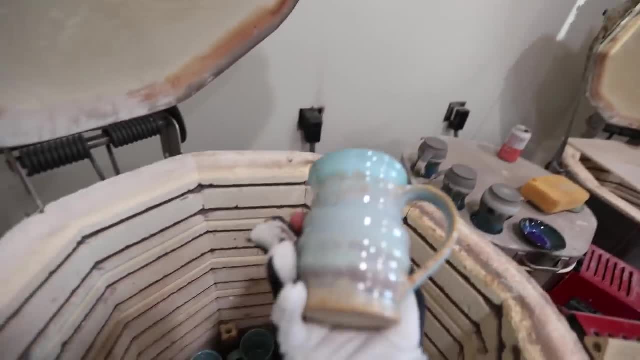 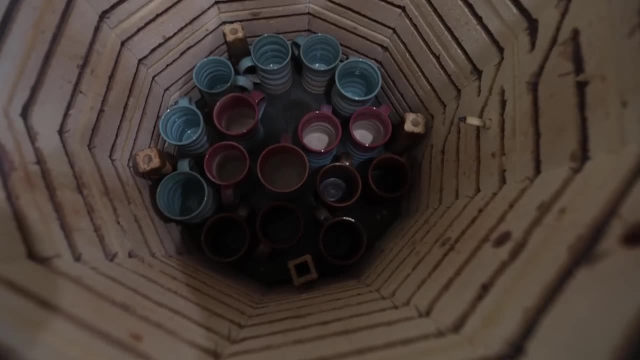 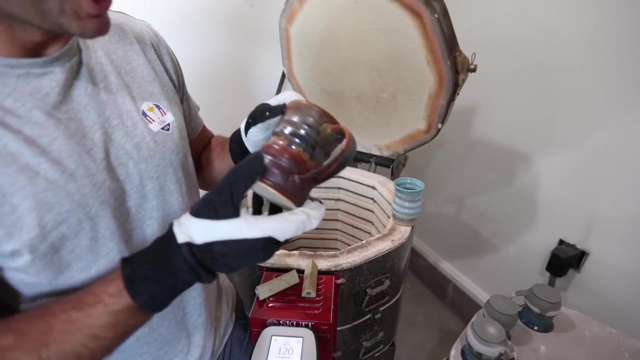 so we got some norse blue Combos. nice, That's beauty. Norse blue over sandstone with not much sandstone showing. Uh, I got some more desert sunsets. noice, Those are big, those are like 20 some ounces. the desert, The desert sunset. 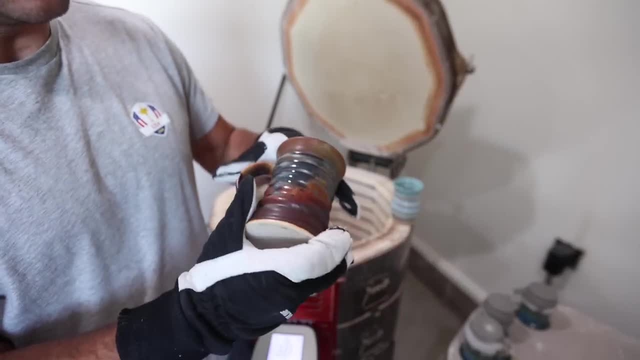 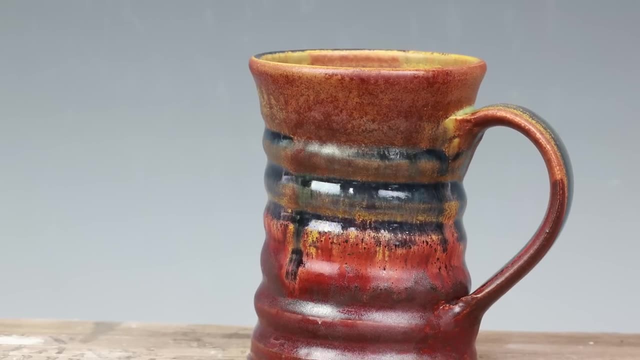 Super happy with that combination. super happy I found it. I love especially- for whatever reason this is happening- where it's matte. It's a matte finish here, So it's not glossy or shiny, and then you get this little section of Glossiness. you know, especially when you you can see it on. 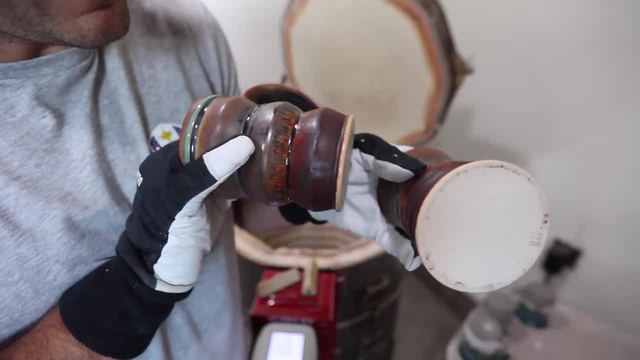 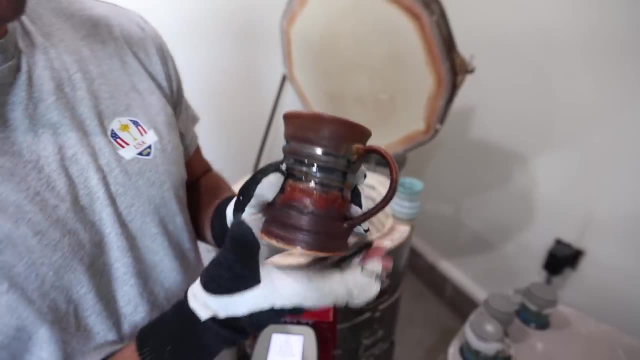 Like these. you get that little section of glossiness, like where the indents are, and that is super cool in my opinion. So you get the mixture in and then it's matte on top. So it's like a matte finish, glossy and then matte. So you get that cool. 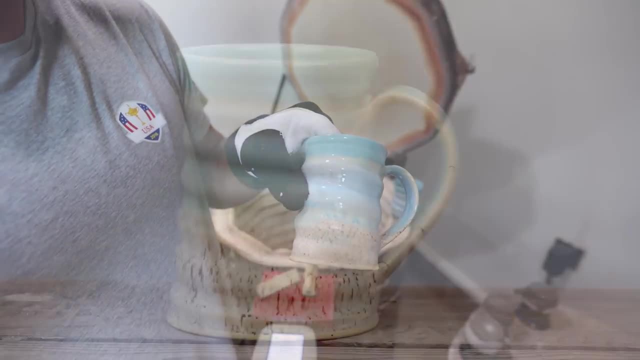 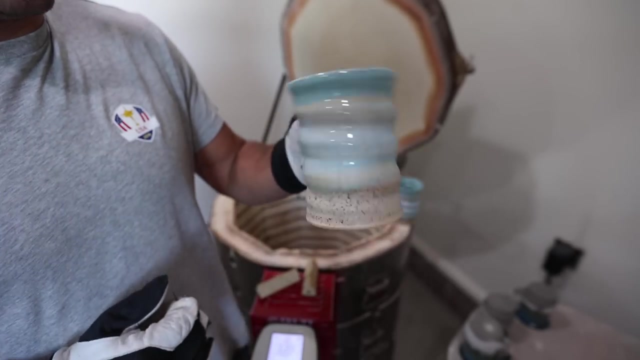 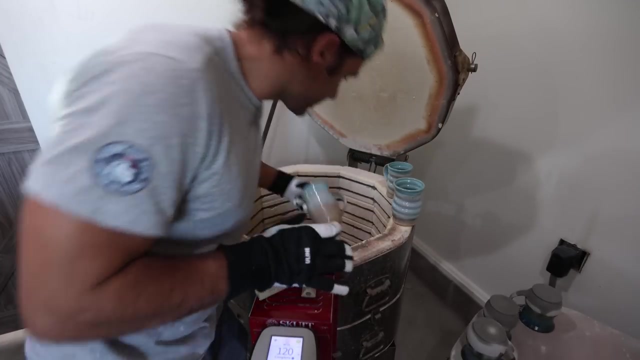 Alright, and then Norse blue and winter wood. I had a few of these kind of testing them out in the restock last month and they all sold really well. this Norse blue and winter wood, and then Sandstone- Wow, we got a few more pink and Norse blue. 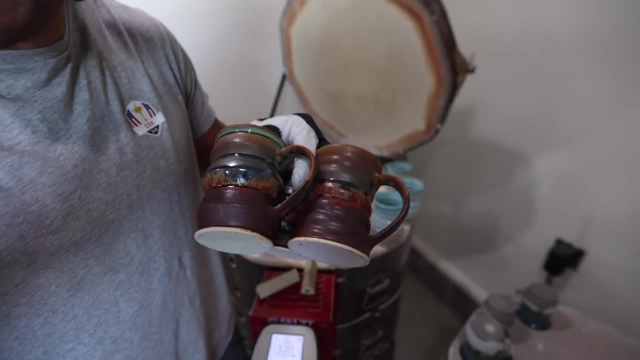 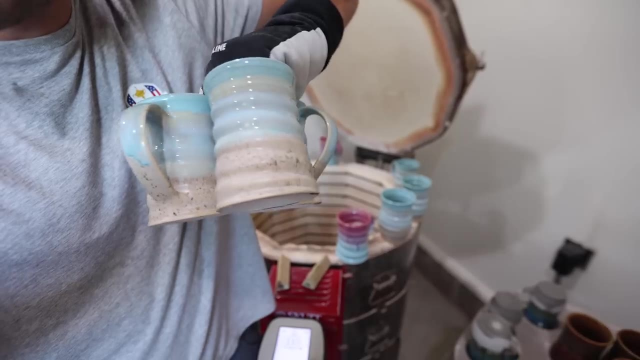 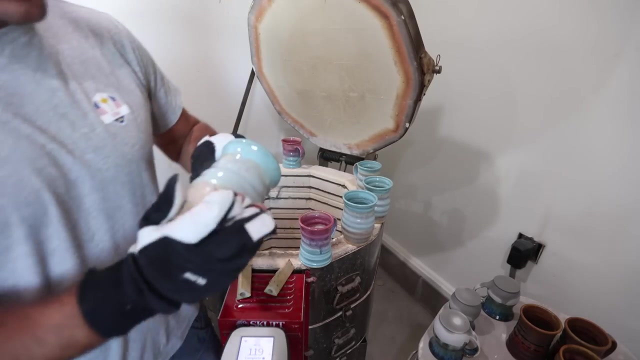 Just so good, I got a turn up, the camera doesn't pick it up. just sweet Norse, blue and winter wood Beauty, full kiln and it's all going up for sale. There we go. All right, There we go. There's the last two. 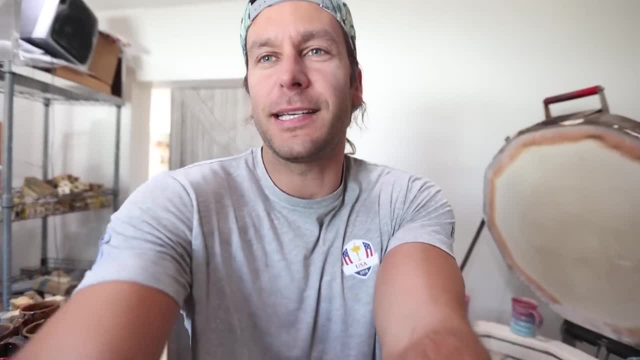 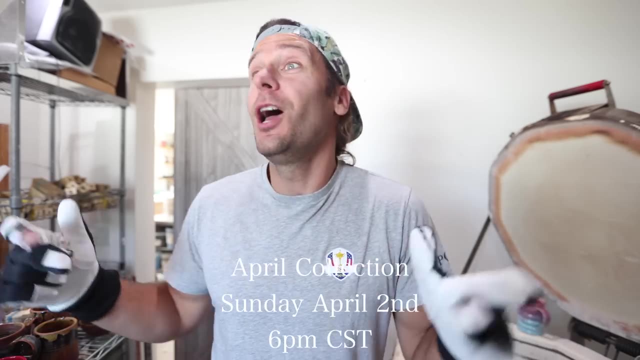 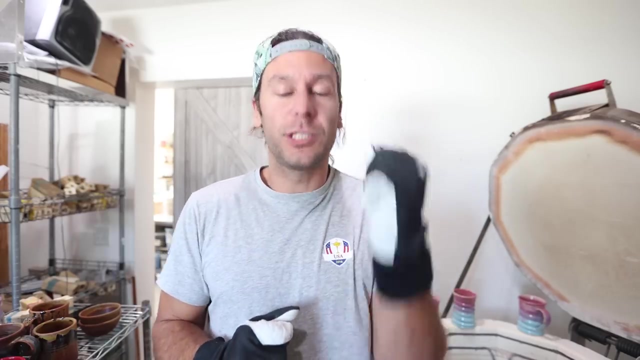 Whoo, all right, that was fun. so I showed you guys exactly how I glaze my best combos. if you want to get any of these, they'll be in the April restock, April 2nd. we have some super exciting things coming. we are getting a gas kiln. yeah, cone 10 reduction. we uh shout out to my 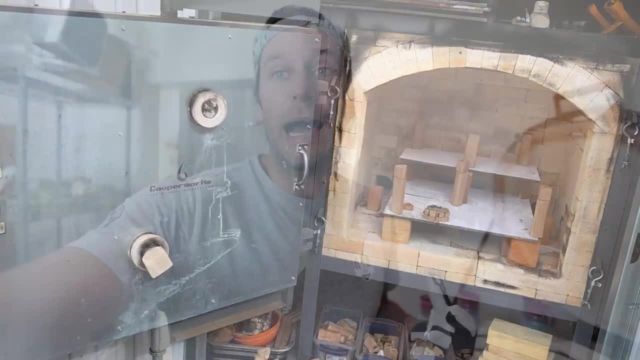 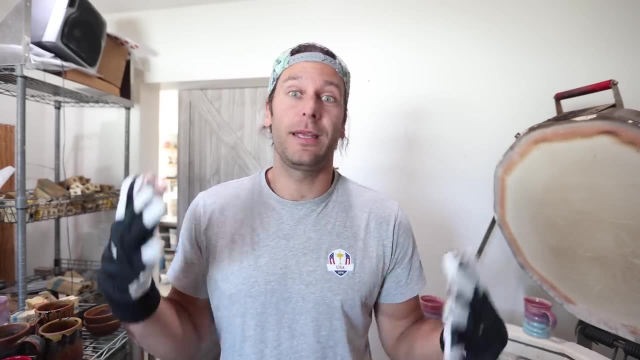 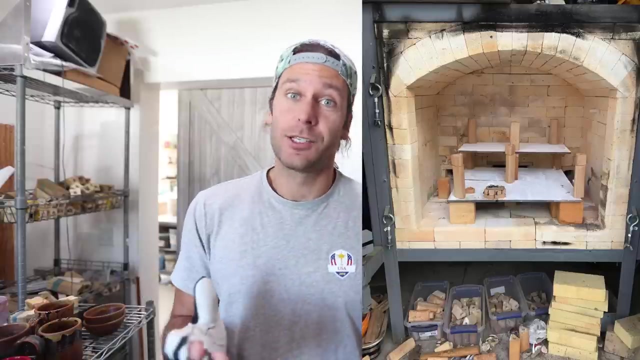 so I'm hiring my intern that I've had the last few years, Kai. so Kai Brisk Pottery, he's worked for me the last few summers. he's graduating, uh, in May and he's gonna come work full-time in the studio with me. so he found a gas kiln in South Dakota for a very good deal, so we are going to go get.